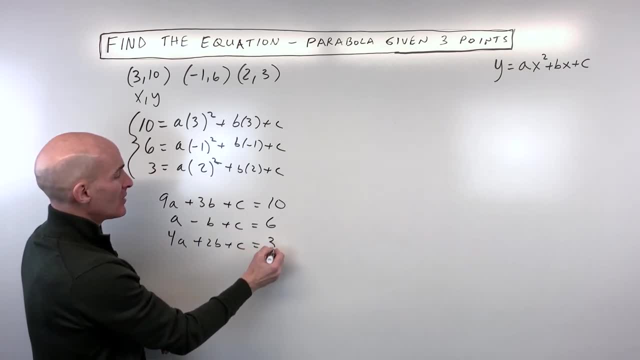 plus c is equal to 3.. Okay, so these are the three variable, three equations that we're going to work with to solve for a, b and c. Now you want to pick a variable to eliminate either the a's, the b's or the c's. 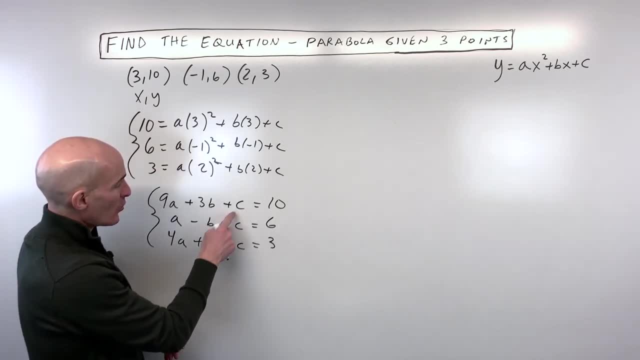 And I'm going to eliminate the c's in this case, because you can see, there's just like one c. it looks like it's going to be pretty easy to eliminate. So what I'm going to do is I'm going to subtract this top equation. 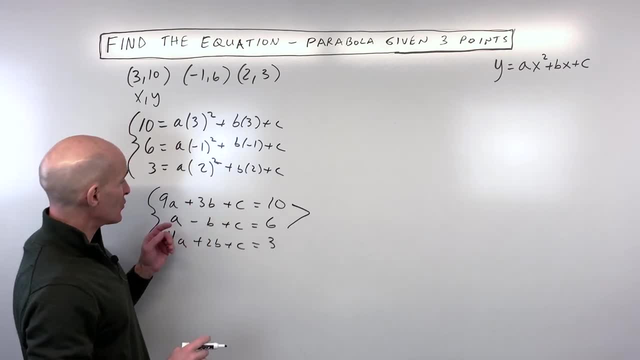 I'm going to take the top equation minus the middle equation, So if I do that, the c's will cancel out. So we have 9a minus 1a, which is equal to 8a. 3b minus negative 1b is 4b, because remember, when you subtract a negative. 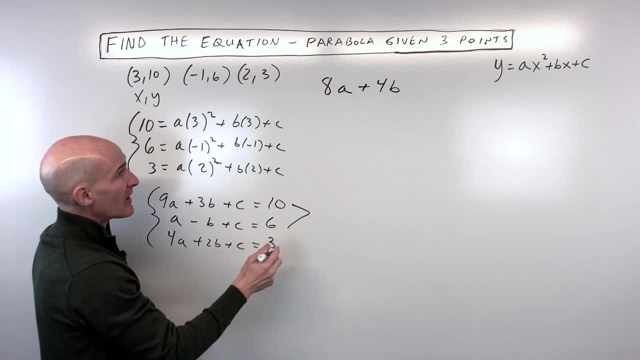 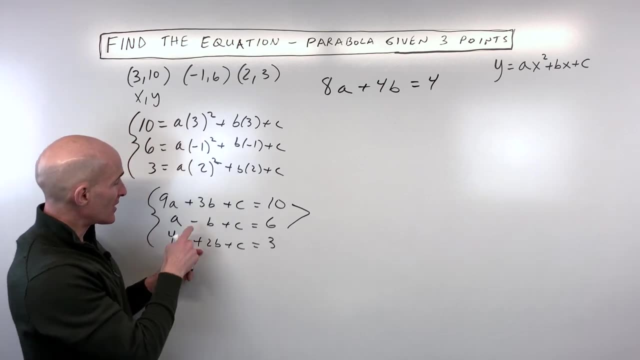 it's like adding the opposite, and c minus c is 0, and 10 minus 6 is equal to 4.. Now we've worked with the first and second equations. now we have to use that third equation. You can either try to combine it with the first or with the second. 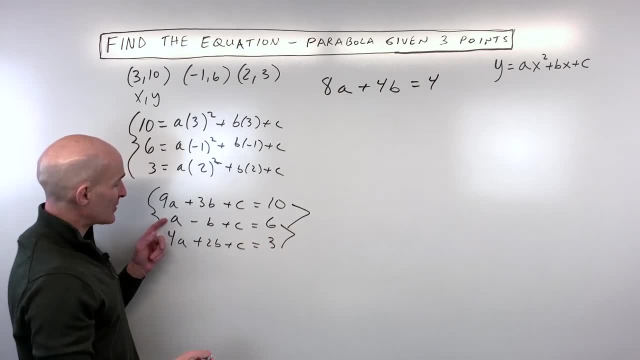 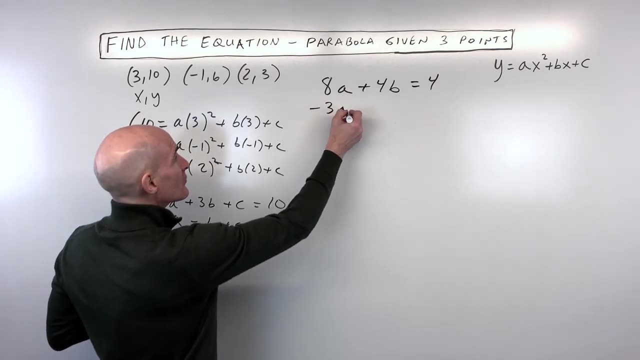 I'll just use the second equation and I'll do that same technique, where I'm going to take the second equation and add it to the third equation. so just subtracting So 1a minus 4a gives us negative 3a. 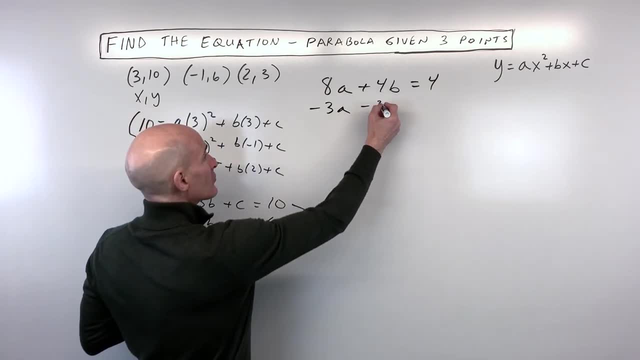 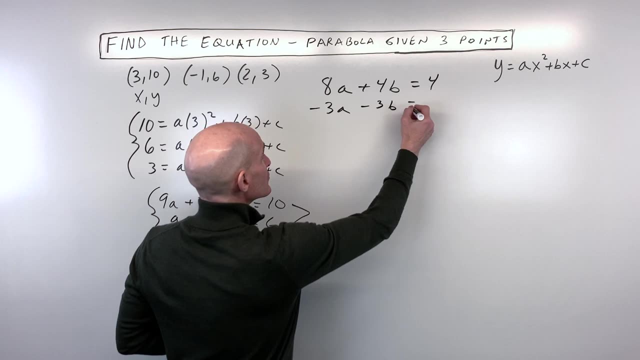 Negative 1b minus 2b gives us negative 3b, And c minus c gives us 0, and 6 minus 3 gives us 3.. Okay, so now look what we have. We have two variables, two equations. 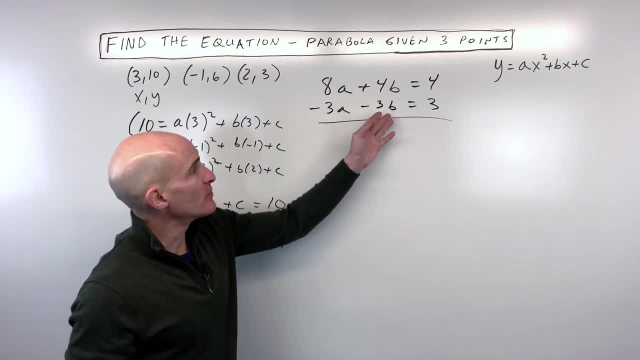 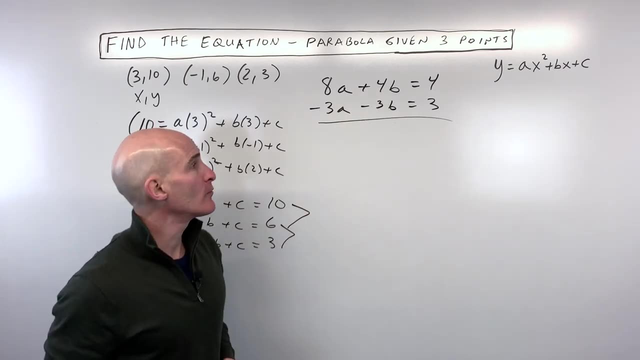 We can solve this system. We need to either eliminate the a's or the b's. I'm going to eliminate the b's, And what we need to do is find the lowest common multiple For 4 and 3.. So what do 4 and 3 both go into? 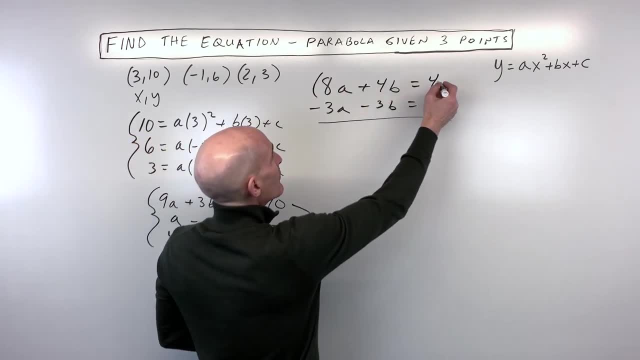 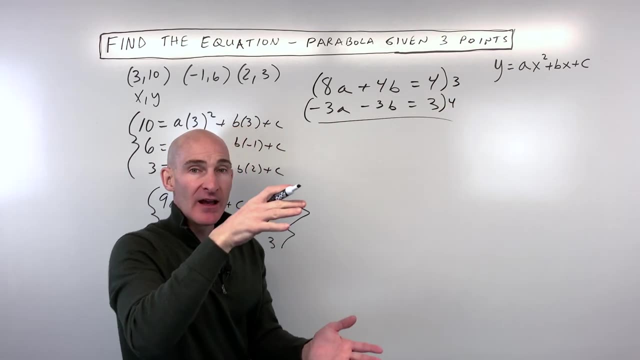 12.. So I'm going to multiply this top equation by 3.. So that'll give us 12b. I'm going to multiply this bottom equation by 4.. That'll give us negative 12b. Then we can add the two equations together to eliminate the b's. 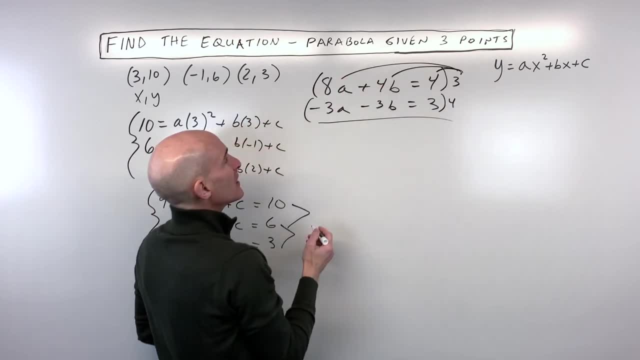 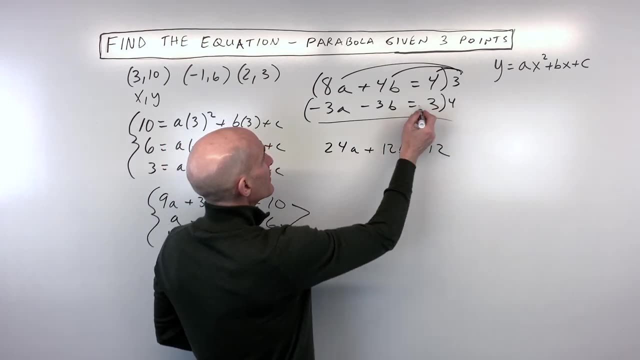 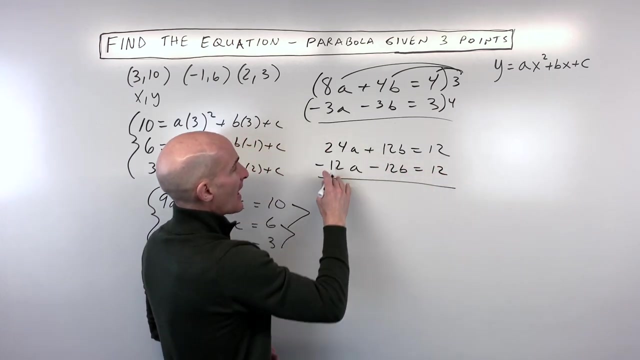 So, first thing, let's just distribute the 3 to the whole equation. Make sure you do it to the left and right sides. Let's multiply this bottom equation by 4.. And now what we can do is we can add straight down. 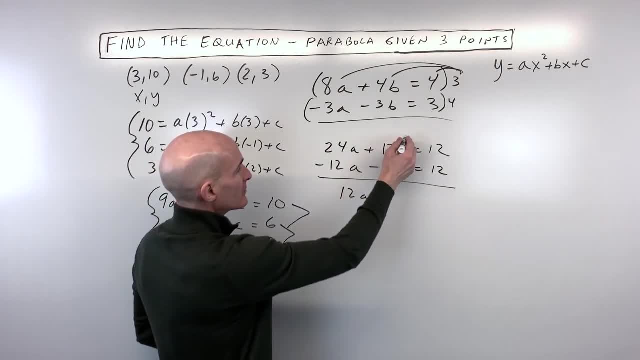 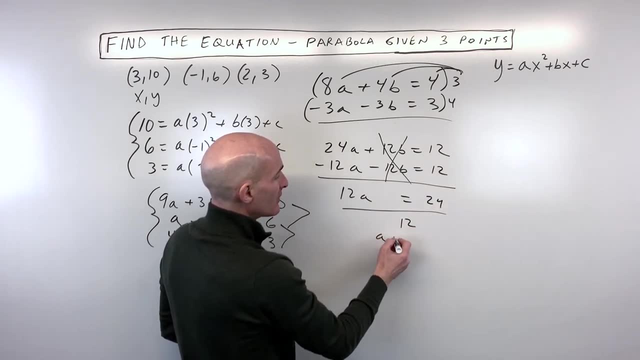 So 24a minus 12a is 12a. The 12b and negative 12b cancel, And 12 plus 12 is 24.. Now if we divide both sides of the equation by 12, you can see we're getting a is equal to 2.. 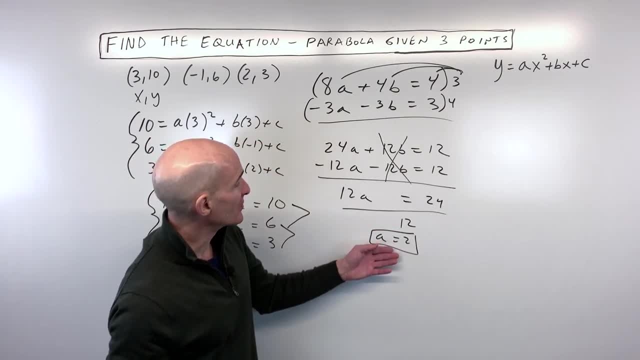 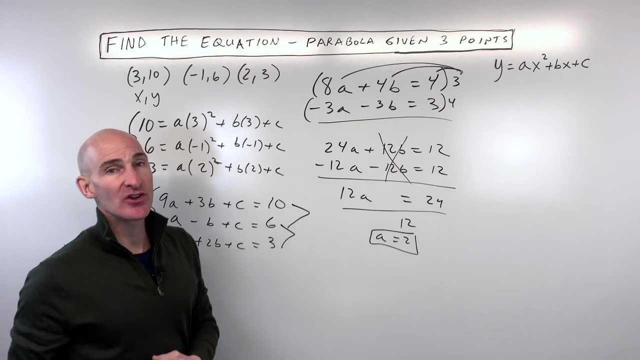 Okay. so now what we're going to do is work our way backwards. We're going to take a equals 2, put it into one of the two variable equations, solve for b, Then go back to one of our three variable equations and solve for c. 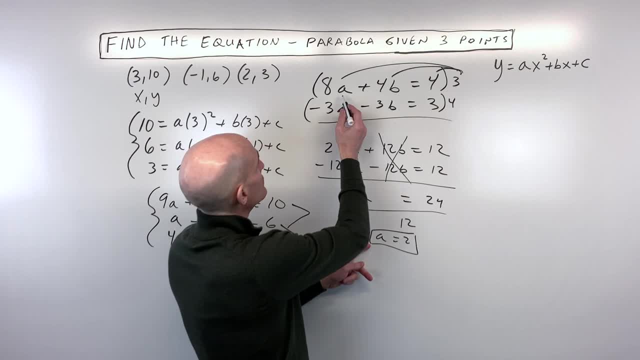 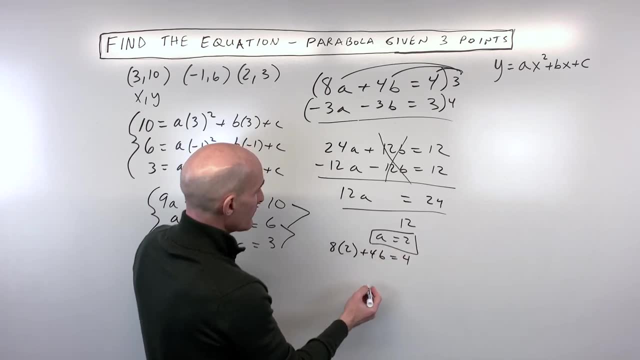 So it's like back substitution. So if we put 2 in, let's put in this top equation, We have 8 times 2 plus 4b equals 4.. So that's 16 plus 4b equals 4.. 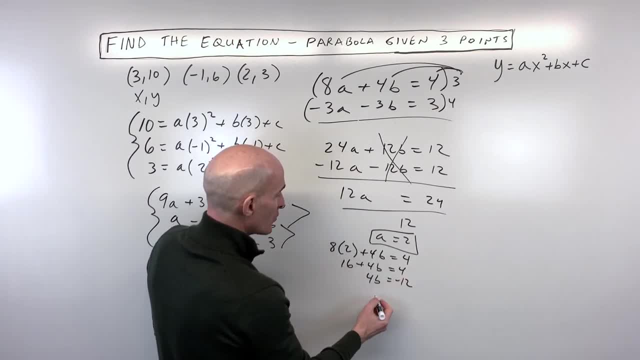 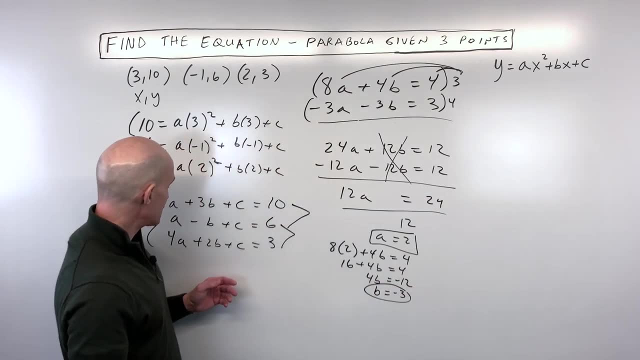 Subtract 16 from both sides, That's negative 12. And divide by 4. You can see we're getting. b is equal to negative 3.. Now we just need to solve for c. Let's see. I think I'm going to use this bottom equation here. 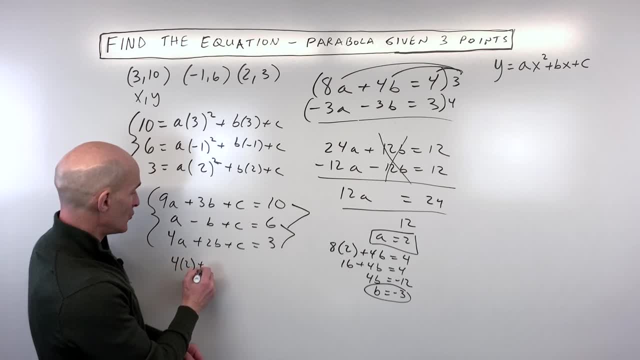 So we have 4 times a, which is 2. Plus 2 times b, which is negative, 3. Plus c equals 3.. Now I could have put it into the first or second equation. I just picked this third one just because I have some space here to write. 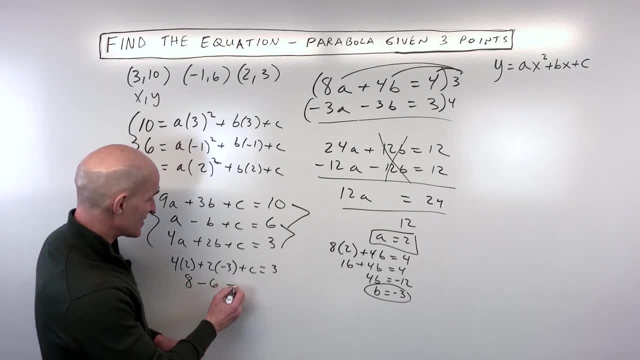 So it would be a little bit easier for us to see. So 8 minus 6 plus c equals 3.. That gives us 2 plus c is equal to 3. And if we subtract 2 from both sides you can see that we're getting c is equal to 1.. 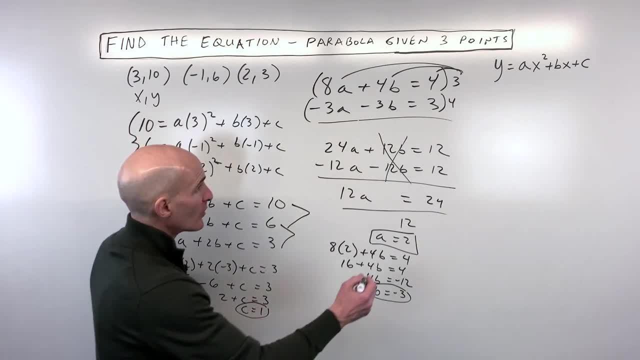 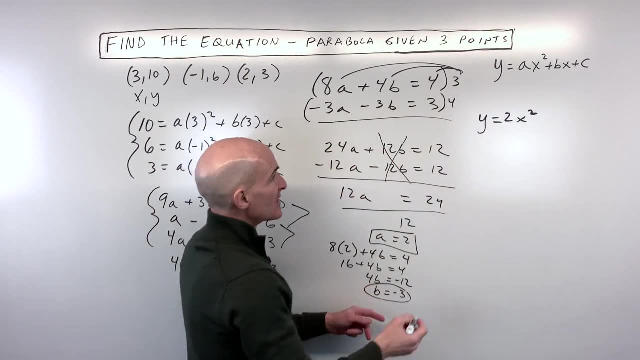 So if we put everything back into our equation there, let's see what we have. We've got: y is equal to a, which is 2. So that's 2x squared. We have b, which is negative 3.. So negative 3x. 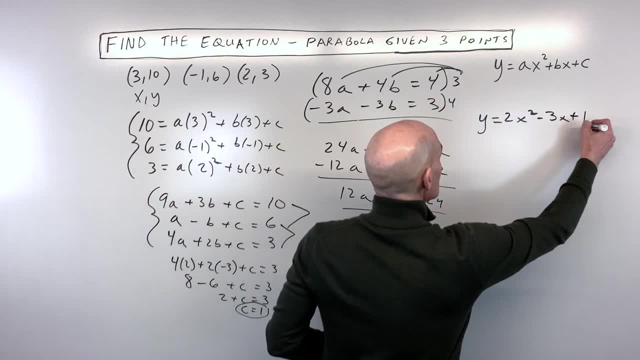 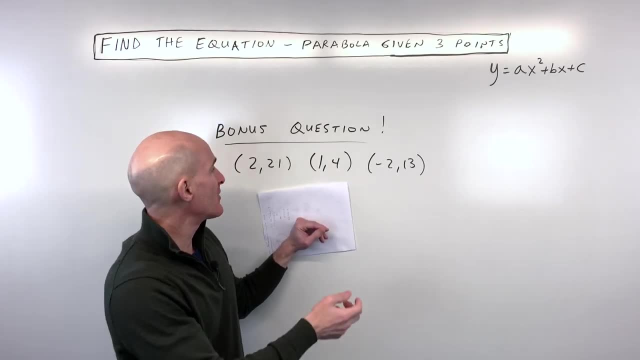 And we have c is equal to 1.. And that's the equation of our parabola, our quadratic. If you'd like some more practice and you want to try one of these on your own, try this one where you have the points 2, 21,, 1, 4, and negative 2, 13.. 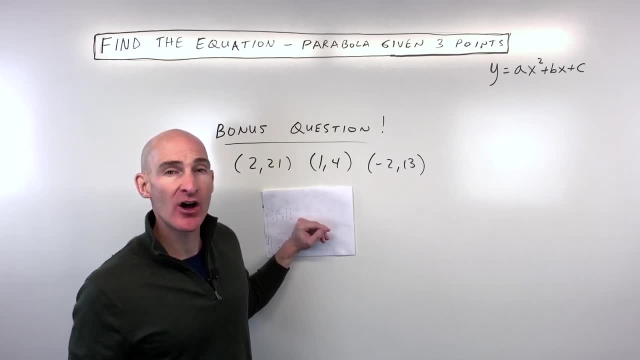 Go ahead and make your system of three variables, three equations, See if you can solve it, And I want to show you the answer here in just a second. But I just want to mention if you're enjoying my content and you want to support the channel.